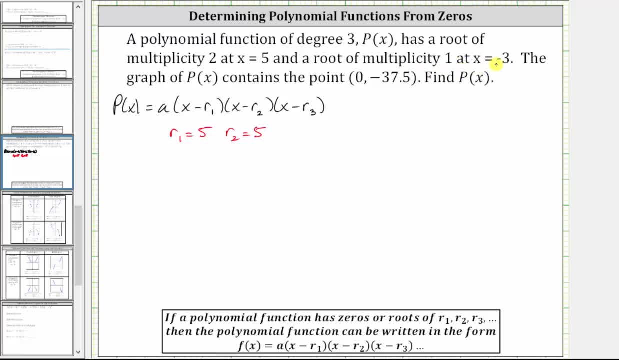 at x equals negative three, which means this is a single root or single zero, and therefore r sub three is equal to negative three. Performing substitution gives us: p of x equals a times the quantity x minus five. times the quantity x minus five. again Notice, because x equals five has multiplicity two. 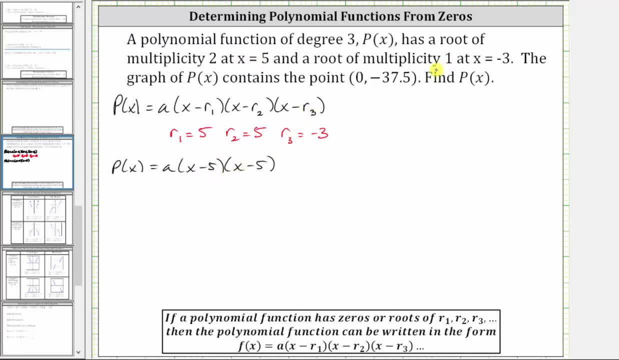 we have two factors of x minus five And then, because the root or zero of x equals negative three, has multiplicity one, we have one factor of x minus negative three. Let's simplify x minus negative three to x plus three. Let's also write this as the quantity x minus five squared. 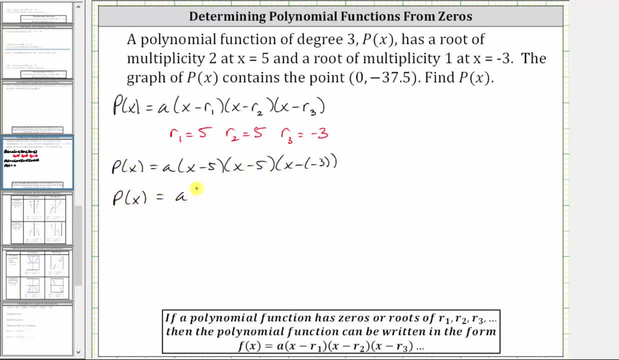 So we know p of x is equal to a times the quantity x minus five, squared times x plus three. Now we need to find the value of a using the given point, which is a vertical or y-intercept, Because we are given the point zero, comma negative 37.5,. 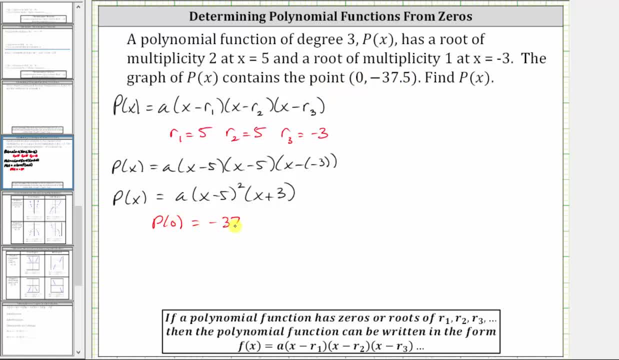 we know that p of zero must equal negative 37.5.. Using this information, we now substitute zero for x and negative 37.5 for the function value here. This will allow us to find the value of a. Performing the substitution gives us negative 37.5. 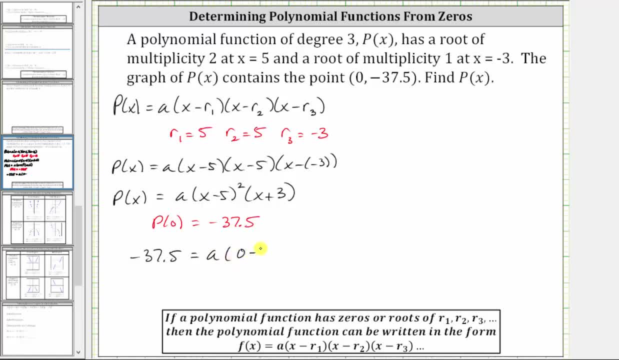 is equal to a times the quantity x minus five. This is the quantity zero minus five squared times the quantity zero plus three. Simplifying, we have: negative 37.5 equals a times the square of negative five, which is 25, times three. 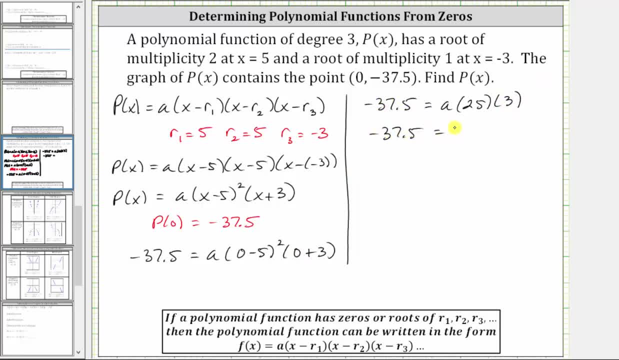 So we have: negative 37.5 equals 75a. To solve for a, we divide both sides by 75.. Simplifying on the right, we have a. a is equal to this quotient here and negative 37.5 divided by 75. 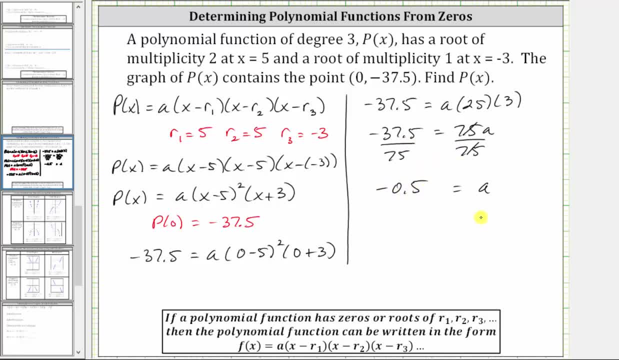 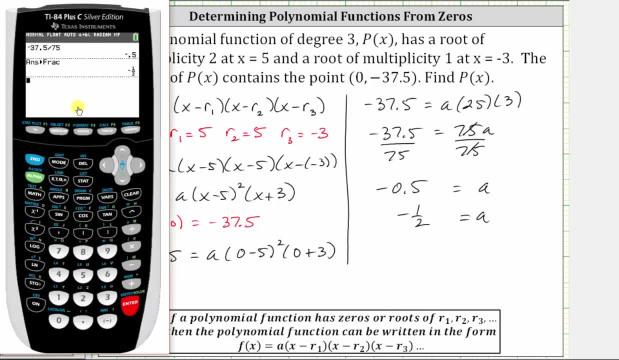 is equal to negative 0.5, or, if we want, negative 1 1⁄2.. Of course, if we needed to, we could check this on the calculator, which I've done here Now that we know the value of a.